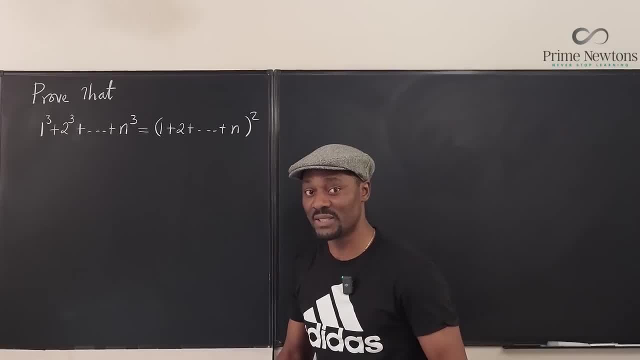 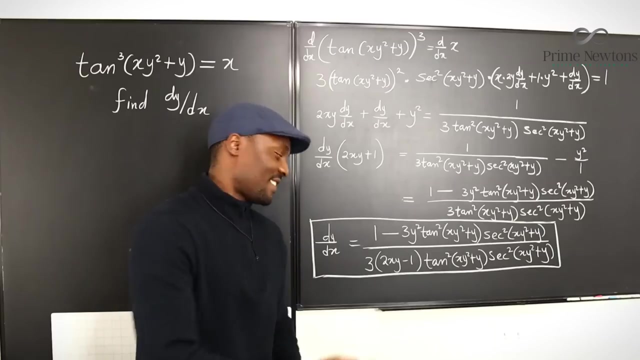 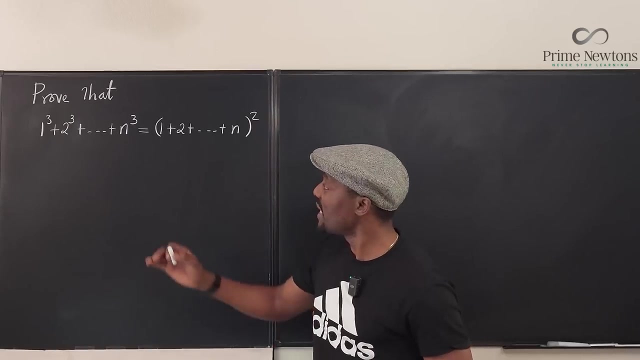 steps that we usually apply when we do mathematical induction, and it's all about algebra and manipulation. when you do mathematical induction and you have to know what you are looking for, Let's get into the video. So the first thing to show is whatever you want to claim. So this is our claim. okay. 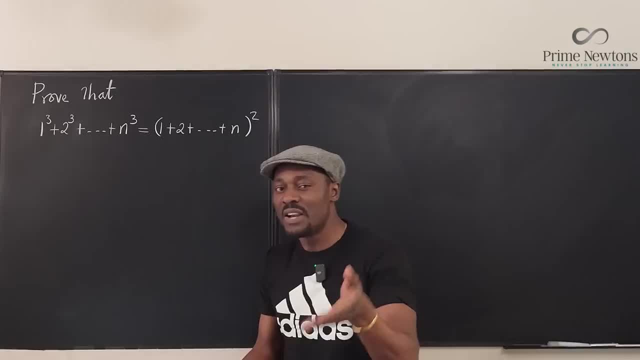 But we have to do some basic tests. We want to test the first number. if it is true, test for maybe another number or maybe a third number, just to make ourselves comfortable with what we're claiming is true, because if you can test it and it happens, you might. 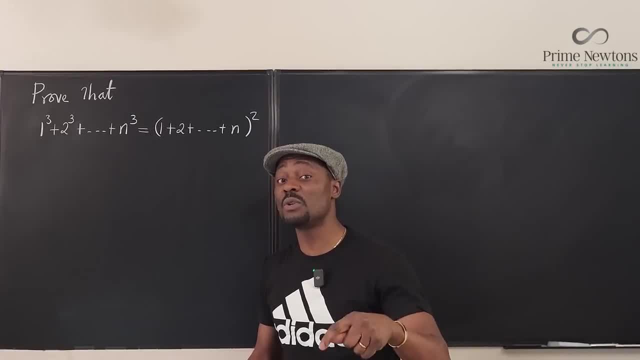 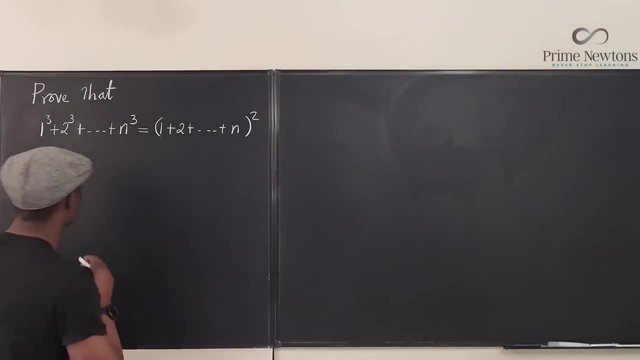 just say: well, it's always true. Well, we want to be able to say: it is always true. and that is the point of mathematical induction. So let's go with the propositions. So we're going to say that the first proposition is: 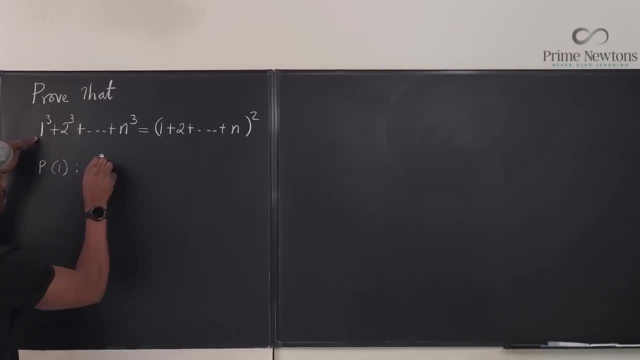 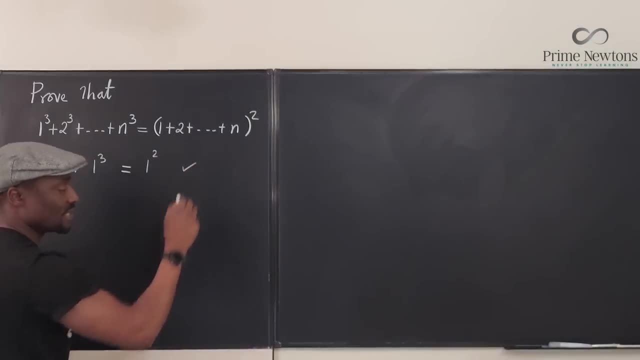 for 1.. We want to claim that 1 cubed will be equal to well, it's just 1, we have 1 squared. Is this true? Yes, this is true, because 1 cubed is 1 and 1 squared is 1.. Well, let's. 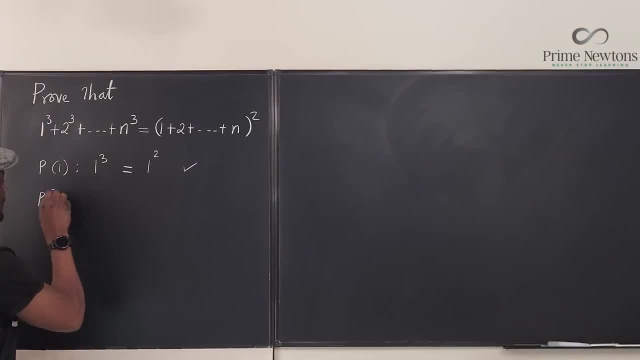 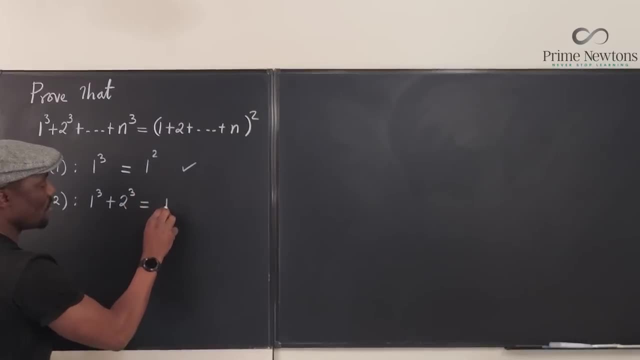 test something else. Let's do the proposition for 2.. We're saying that 1 cubed plus 2 is 2 cubed will be equal to 1 plus 2 squared. Is this true? Well, 1 cubed plus 2 cubed is. 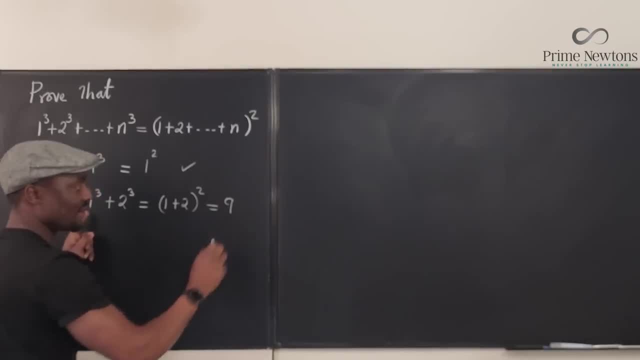 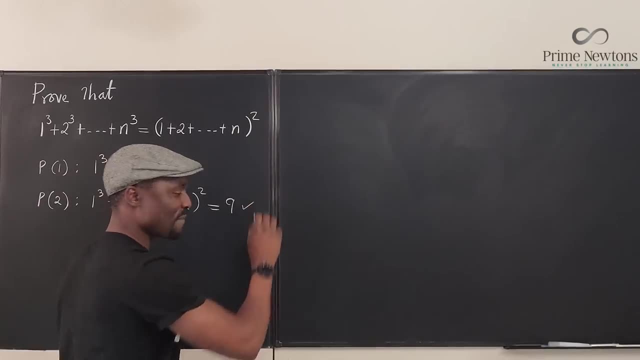 9.. 1 plus 2 is 3.. 3 squared is also 9.. See, it's 1 plus 8.. This is true. Let's test one more. Okay, let's do proposition for 3.. It will be such that we have 1 cubed plus 2 squared. 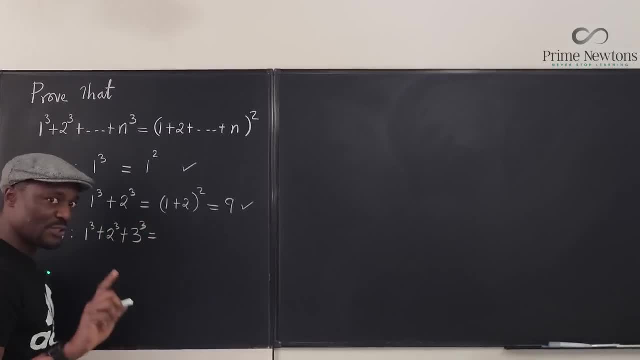 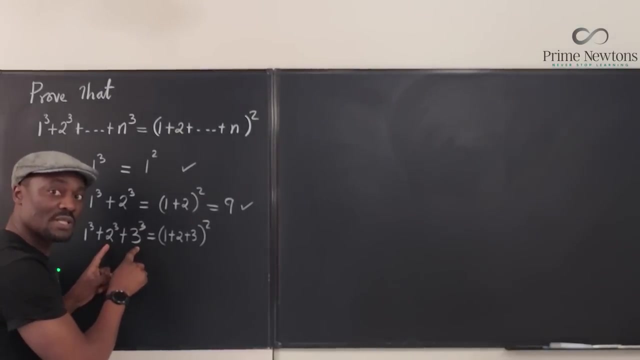 plus 3 cubed, Is it true that this will be equal to 1 plus 2 plus 3 squared? Let's see: This is 1 plus 8.. That is 9.. 3 cubed is 27.. 27 plus 9 is 36. And this is 6 squared. It's. 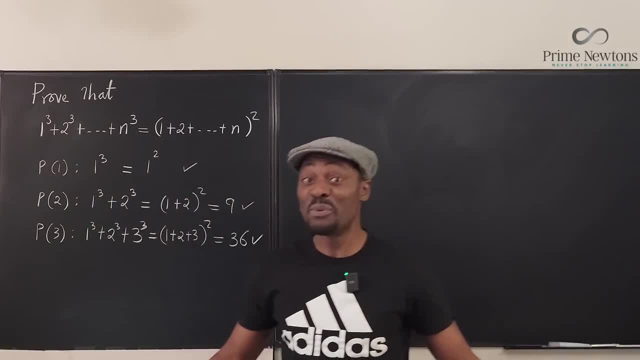 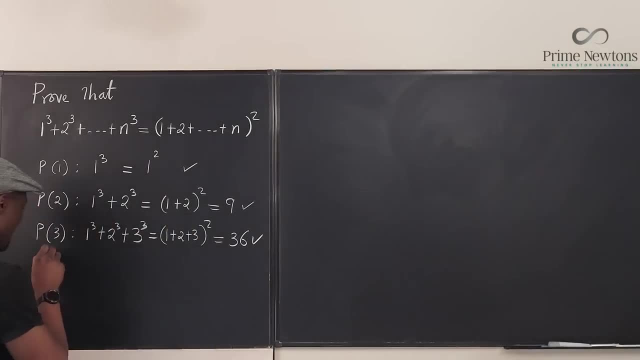 36.. So it looks like it will always happen, but we don't know that. We need to prove it by mathematical induction. So what we're going to do now is we're going to keep going, and so we're going to assume it is true, for n is equal to k. Okay, Maybe I should have been. 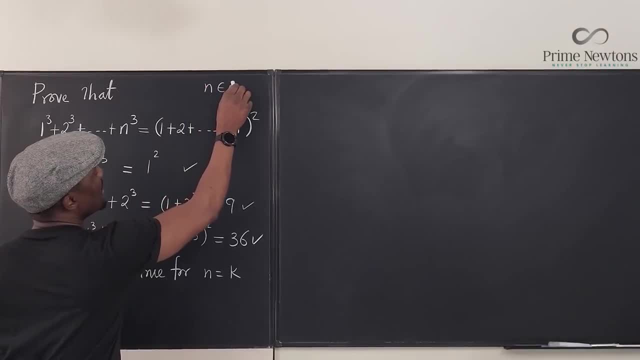 writing. n equals k. By the way, n must be a natural number, That is, we'll start from 1, 2, 3, 4,, 5, 6, 7,, 8, 9,, 10,, 11,, 12,, 13,, 14,, 15,, 16,, 17,, 18,, 19,, 20,, 21,, 22,, 23,, 24,, 25,. 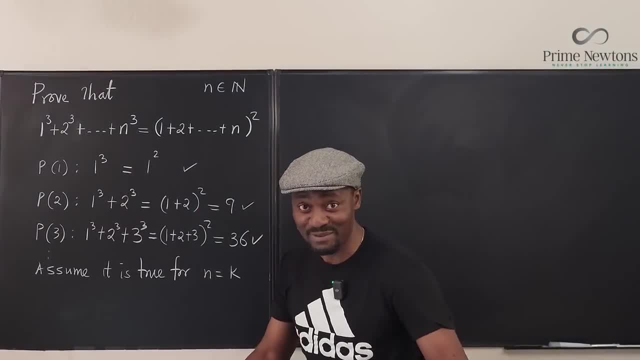 26,, 27,, 28,, 29,, 30,, 32,, 33,, 34,, those numbers like that. We're not talking about fractions or negative numbers. Okay, Just natural numbers Now. so let's assume it's true for k then. 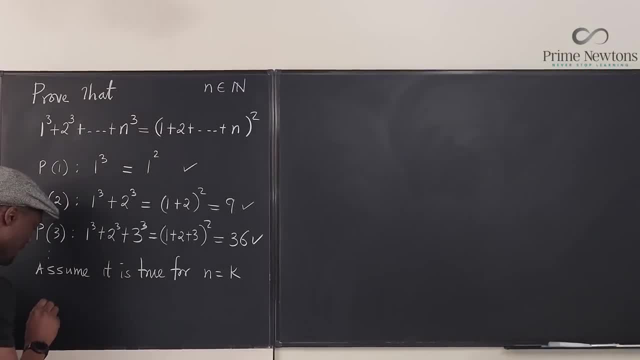 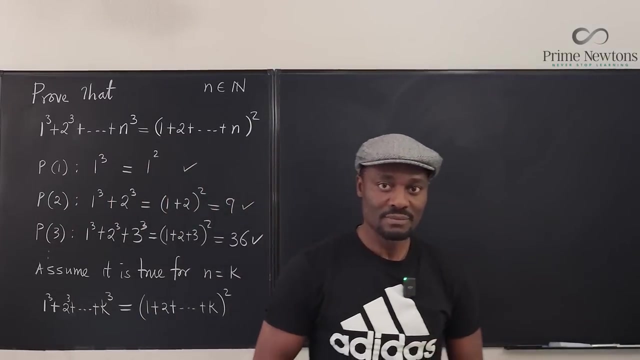 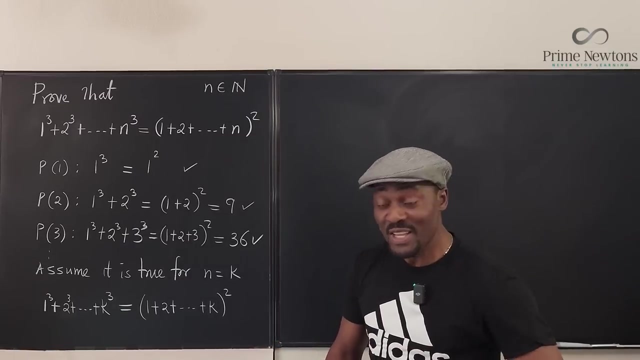 it means we can write this and say that: 1 plus 2 plus, if we cube each of them, we're claiming that this will be equal to 1 plus 2 plus k squared. Thank you, squared. so what do we do next? we don't need to show that it is true if you go. 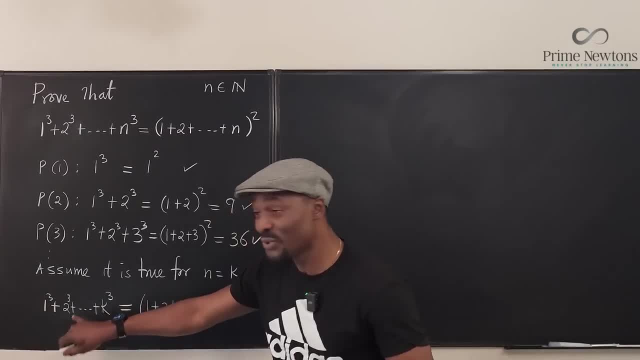 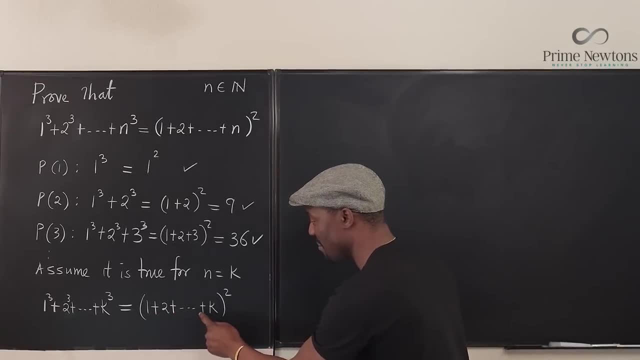 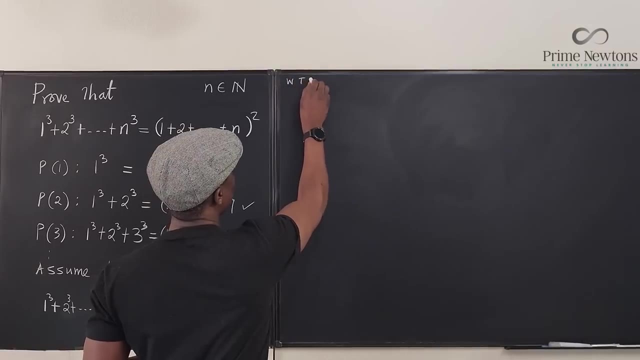 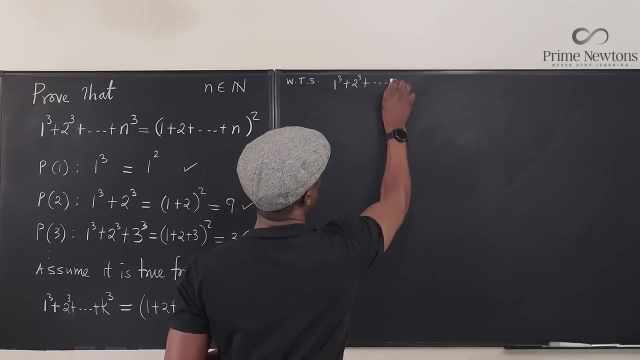 one more step. we want to show our 1 cube plus 2 cubed plus tap, tap, tap plus K cubed plus K plus 1 cubed will be 1 plus 2 plus blah, blah, blah plus K plus K plus 1, squared, okay. so we want to show, want to show that 1 cubed plus 2 cubed plus K. 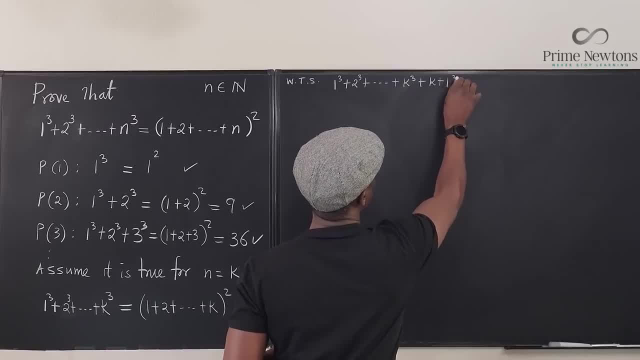 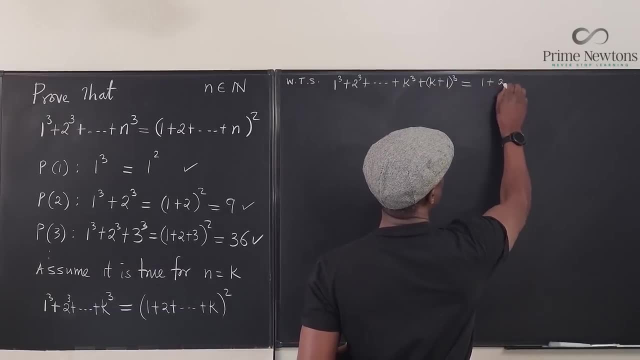 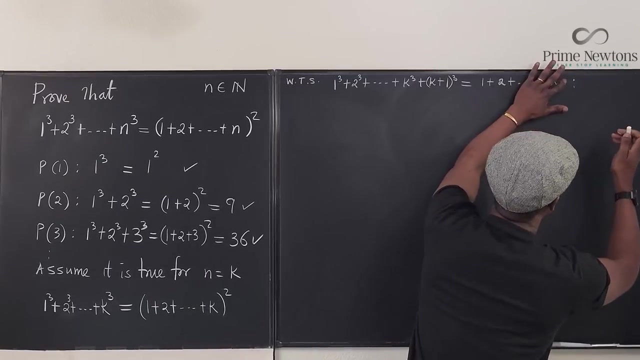 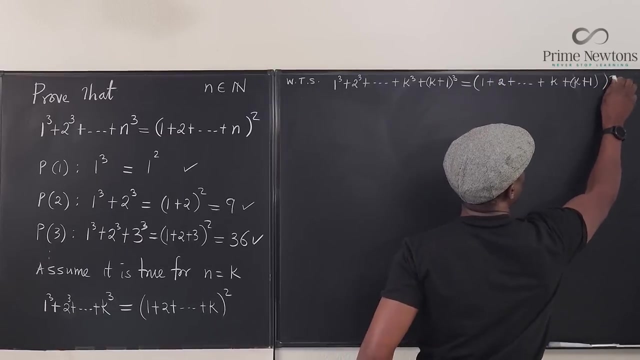 cubed plus K plus 1 cubed. this is what we want to show. okay, K plus 1 cubed is equal to 1 plus 2 plus K plus 1, sorry plus 2 k. okay plus k plus one, everything squared. this is the claim. if we can do this, then we're correct. 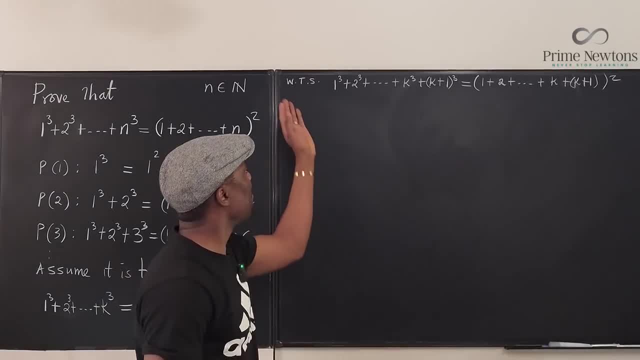 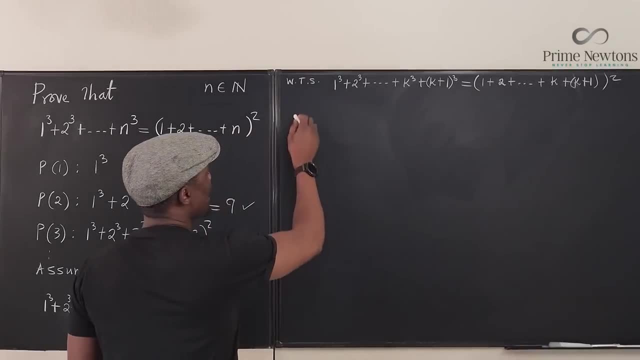 okay, what should we do? well, we have to start from the left hand side. we want to show that we're going to get this at the end. okay, in the end. so here we have p of k plus one using. so this is what we want to show: we're going to get this at the end. so let me just rule that. 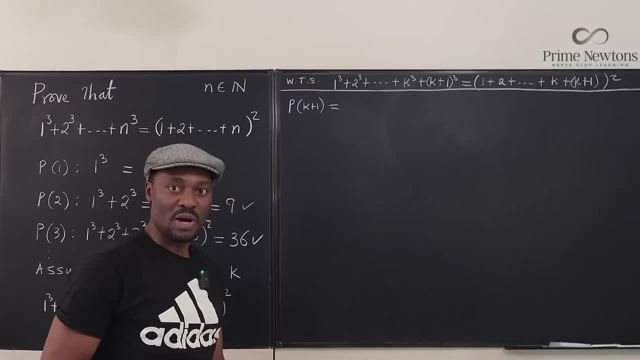 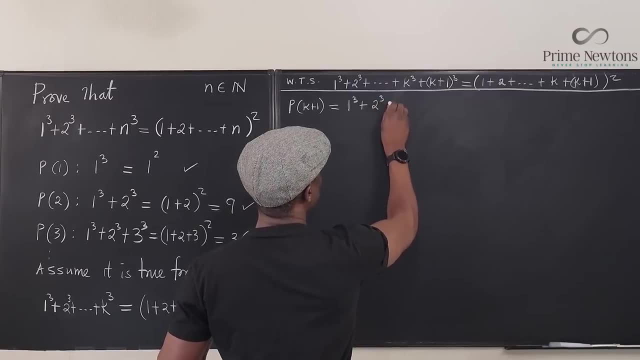 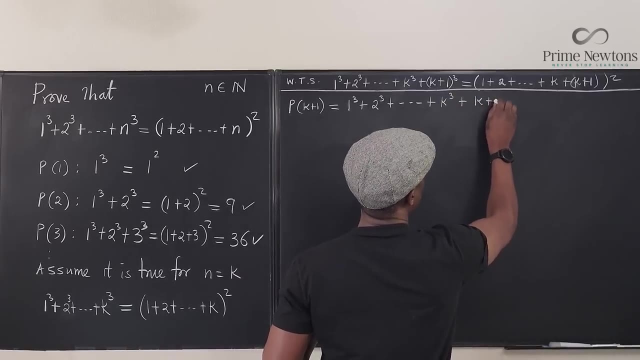 out. okay, now, p of k plus one, following this rule, is going to be one cubed plus two cubed plus plus k cubed plus k plus one cubed. right, but the claim we're saying we're saying is that we're going to get this at the end, so let me just rule that out. 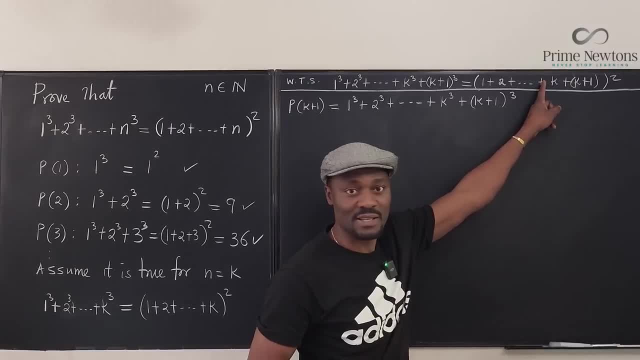 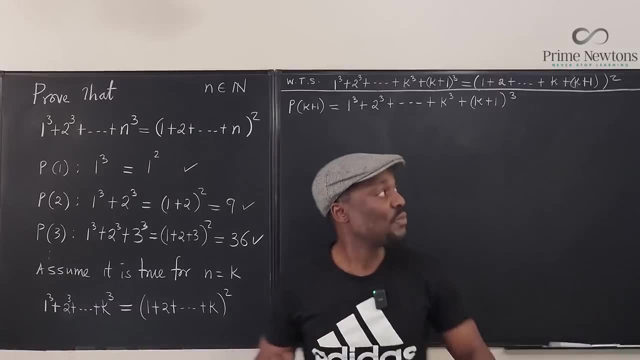 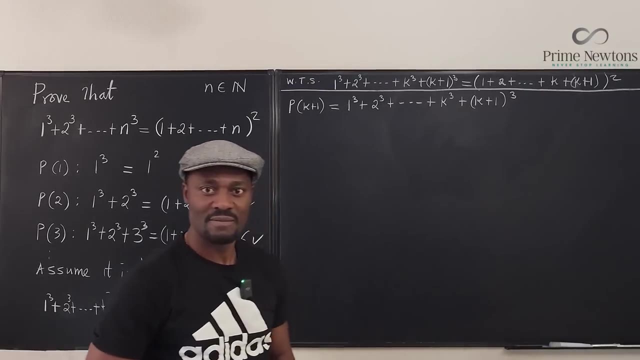 we have right now is that what i just wrote is the same thing as this. okay, it's just an extension of this. if we put k plus one inside, just add k plus one, because, since that is the last term, so how can we make this look like that? now watch this. this is a strategy you want to adopt in a 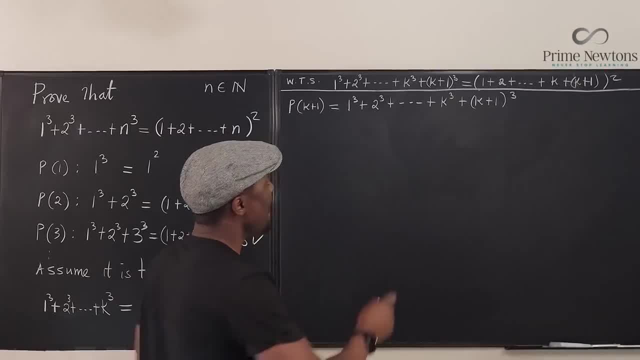 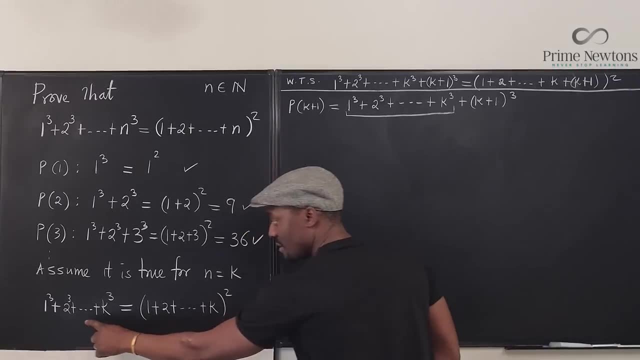 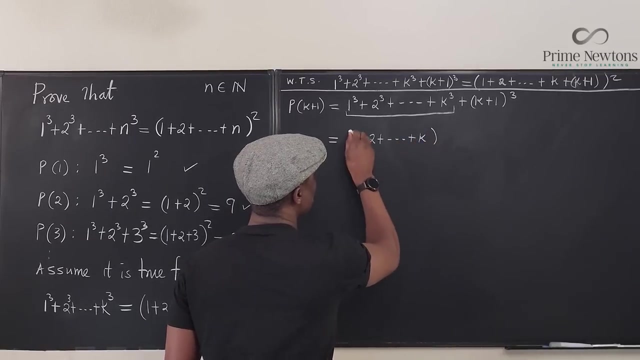 case like this, when you're doing a series. okay, look at the first set of terms here. we already claimed here that this is equal to this. that means i can repeat this and write this instead. i can write one plus two, plus top, top, top, plus k, and i'm going to write squared plus k, plus. 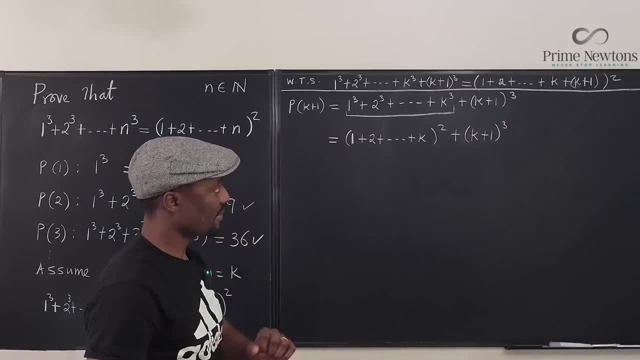 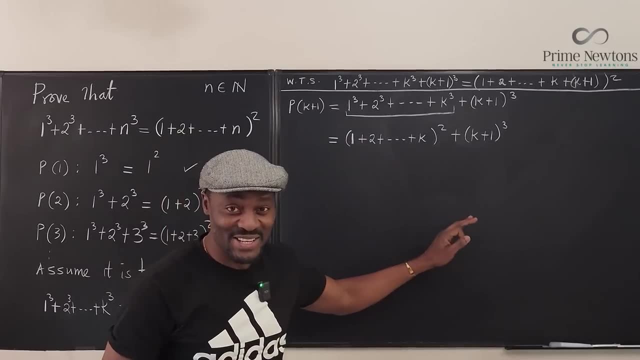 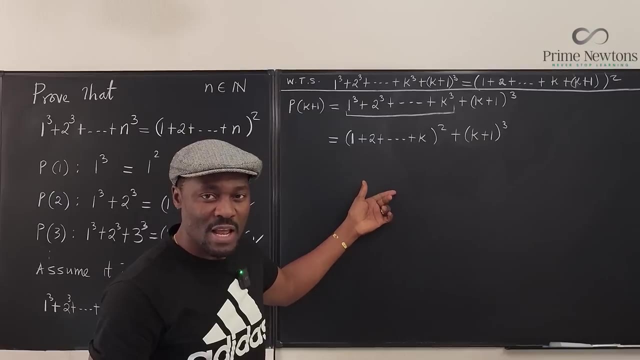 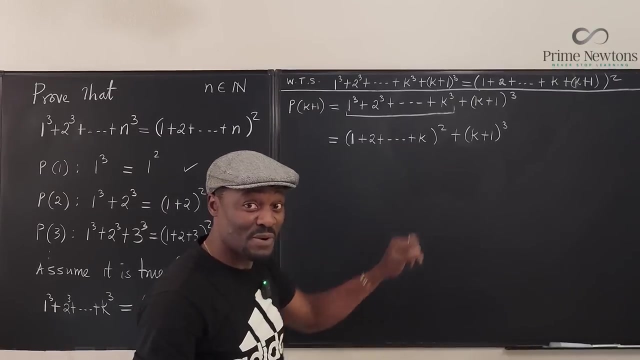 one cubed. okay. now the problem with the problem, with the problem with mathematical induction is you're expected to know something else that is easier than what you're doing. do we know the sum of the first k terms? yeah, the sum of the first n terms. look: one plus two plus. 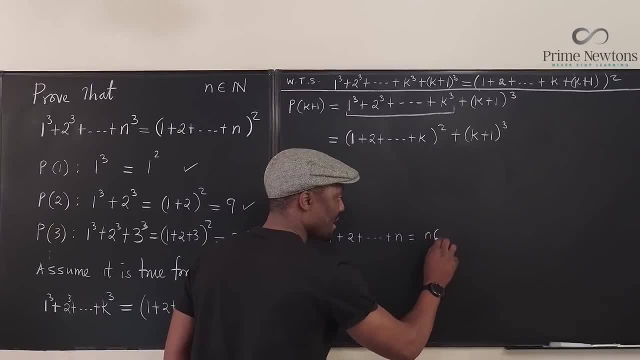 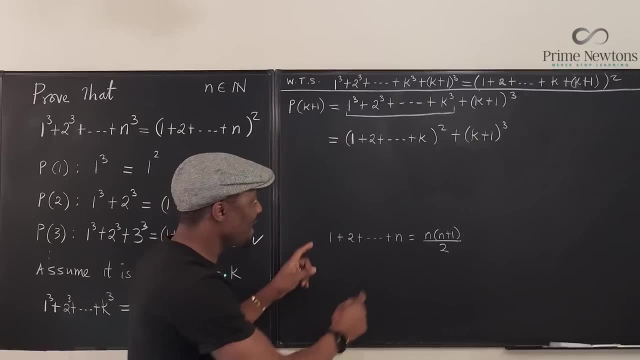 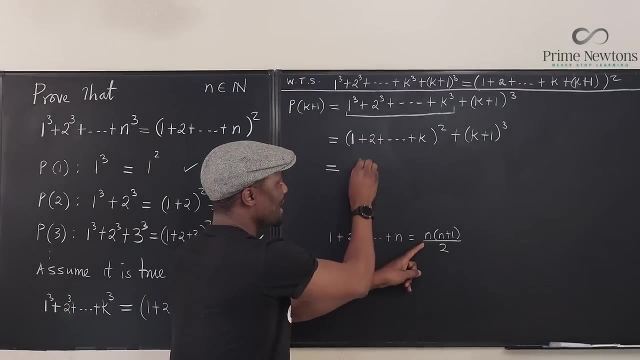 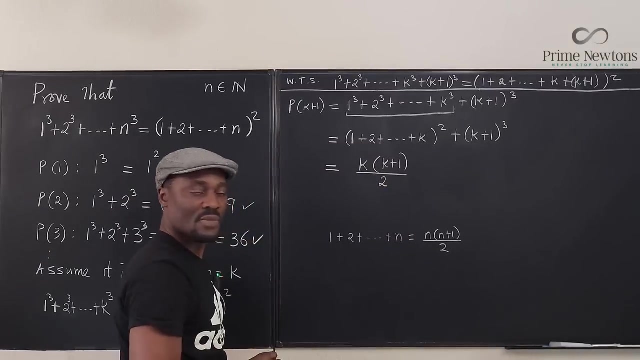 n has a formula. it is basically n times n plus one divided by two. do you remember this formula? yes, so we could. instead of writing this long chain, we could actually write this as: instead of writing this, we could write this as: k times k plus one over two. but this is going to be squared because 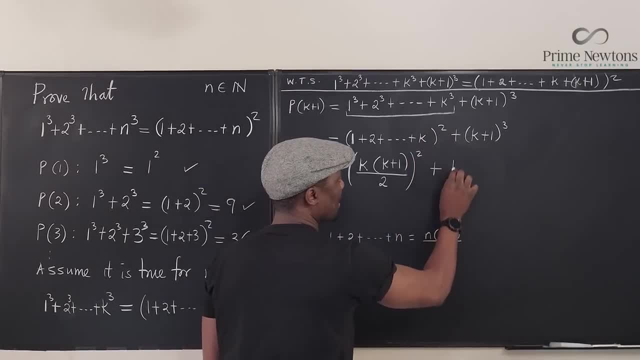 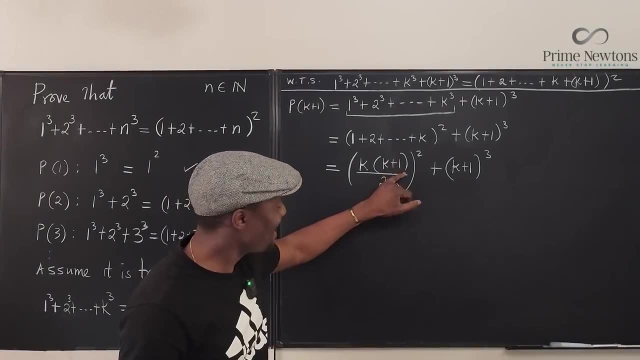 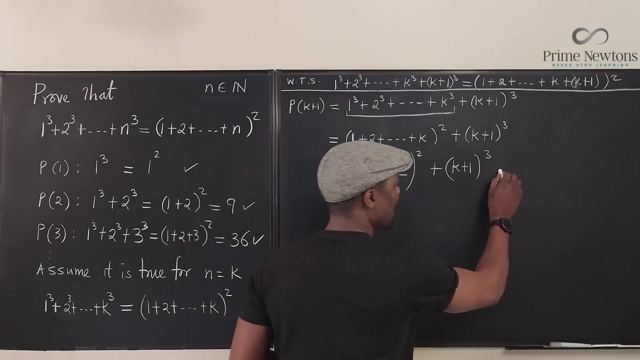 this is squared plus k plus one cubed. let's get rid of this. now you can see that we have k plus one here. we also have k plus one here, so the opportunity to factor is beginning to show up, right, okay, um, let me see, let me go this way. i'm going to simplify this and write this as: 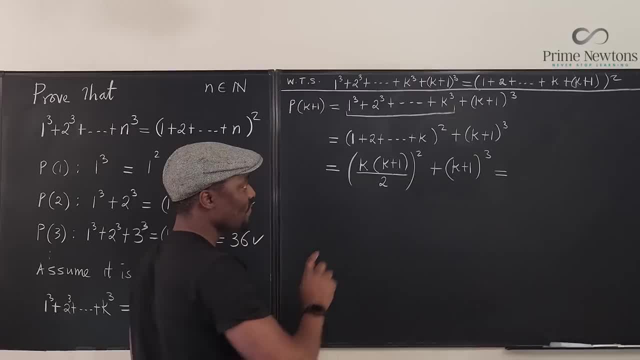 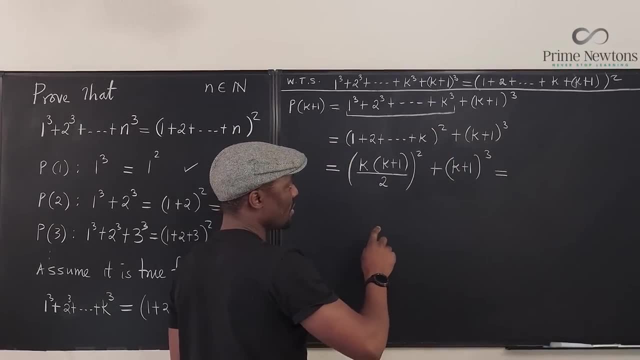 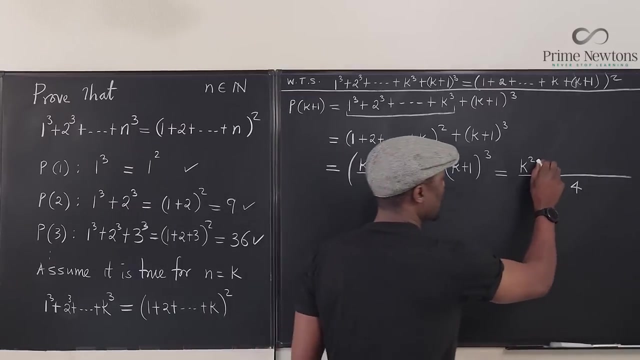 this is going to be k squared, k plus 1 squared, k plus 1. cubed over. i can put all of these under the same um, so let's do this. so i'm going to square this. this is going to be 4. i'm going to square this. this is going to be k squared. this would be k plus 1 squared. 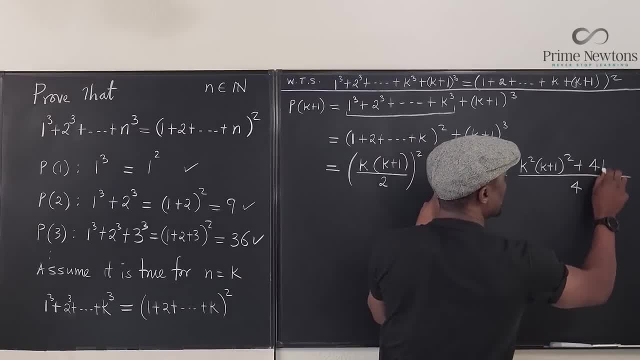 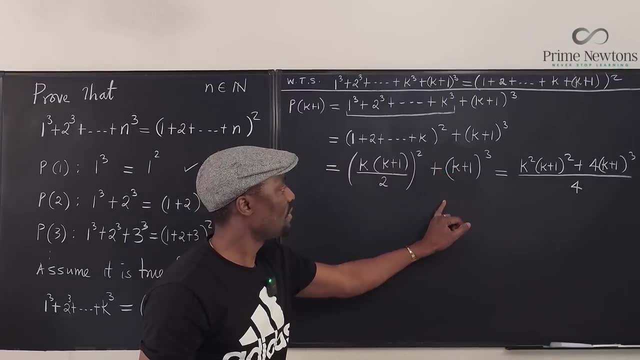 and i'm going to write this as plus 4 k plus 1 cubed. now, why is this 4 k plus 1 cubed? i just wrote this as 4 over 4, okay, so that the two will have the common denominator. let's clean this up. 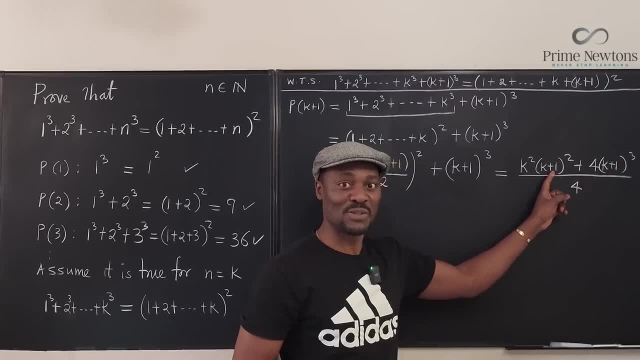 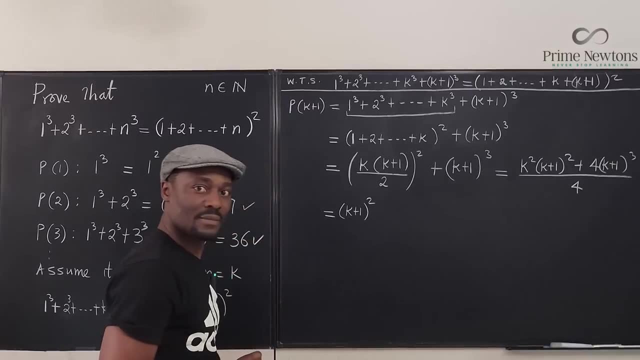 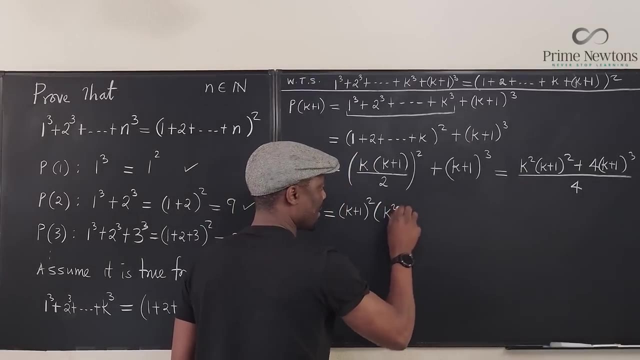 what is common to this term and this term? k plus 1 squared. i'm going to pull it out. so i have k plus 1 squared. nice, and what is left? i've got k squared. and what is left here? i got four. oh, i got four times. 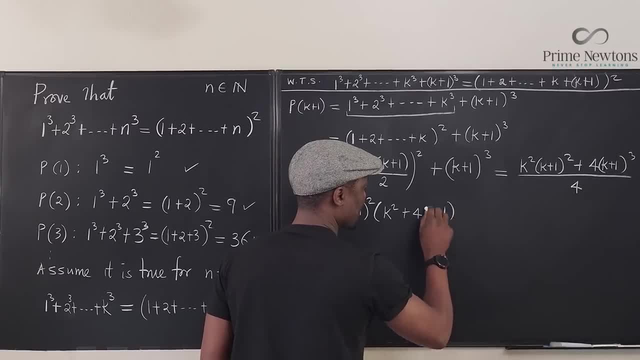 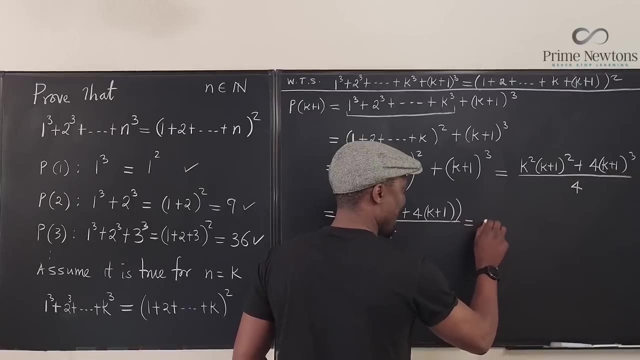 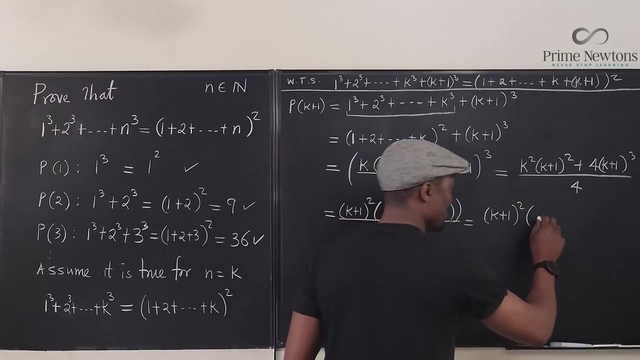 k plus one, right, or i can actually. okay, let's leave it this way and everything is divided by four. but pay close attention, this is the same thing as k plus 1 squared times. if you distribute this, it's going to be k squared plus 4k.